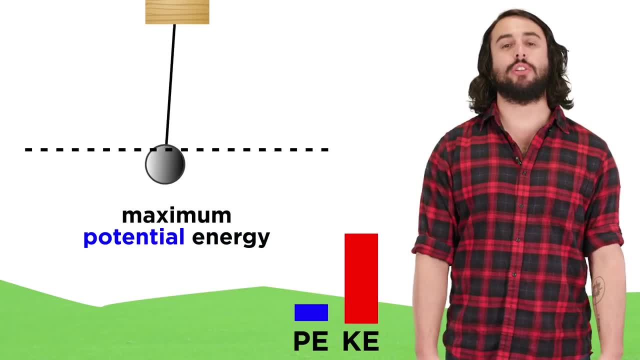 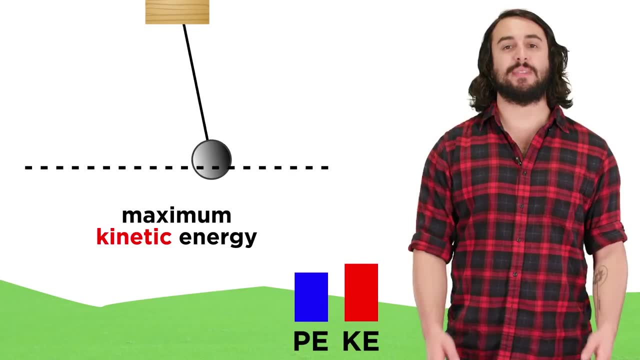 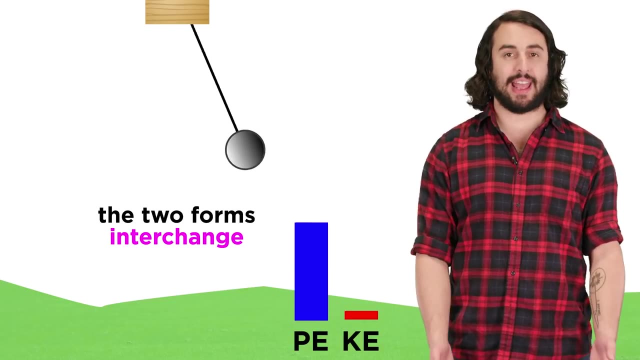 energy. At the top of the swing, the pendulum possesses its maximum potential energy and zero kinetic energy. At the very bottom of the swing, it possesses its minimum potential energy and its maximum kinetic energy. As these two forms interchange again and again and again, there is conservation of energy. 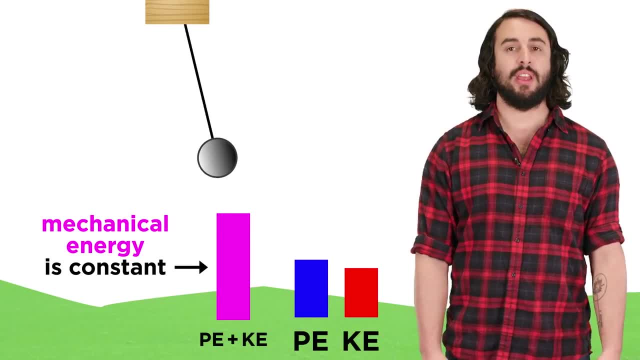 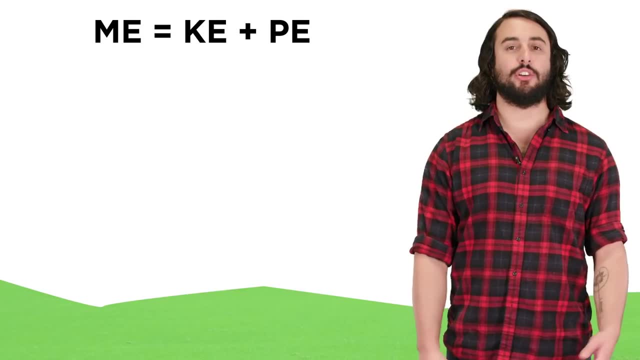 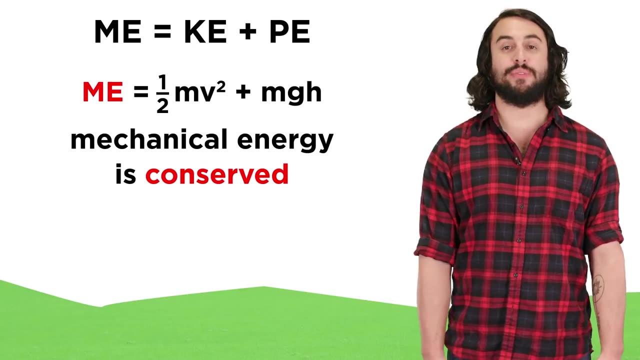 and the total mechanical energy, which again is the sum of the two, is constant. This concept can be described mathematically by the following equation: If mechanical energy is the sum of kinetic energy and potential energy, which are in turn represented by these expressions, and this value is conserved, then one half mv-squared. 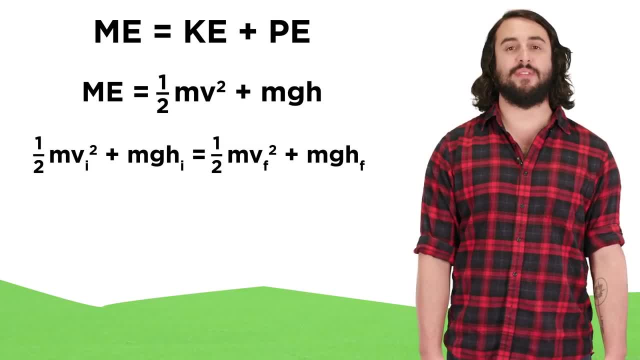 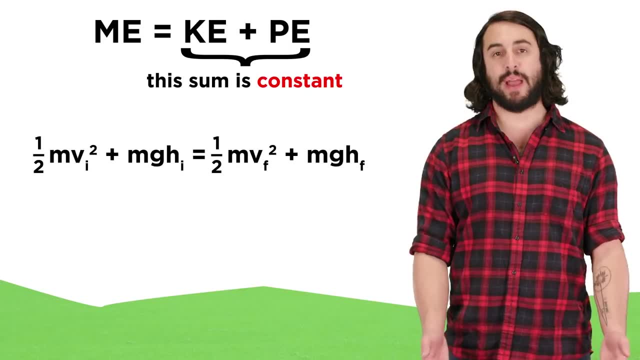 initial plus mgh initial will be equal to one half mv-squared final plus mgh final. It shows that the sum of the kinetic and potential energies of a system like the pendulum will be the same at every point in its motion. 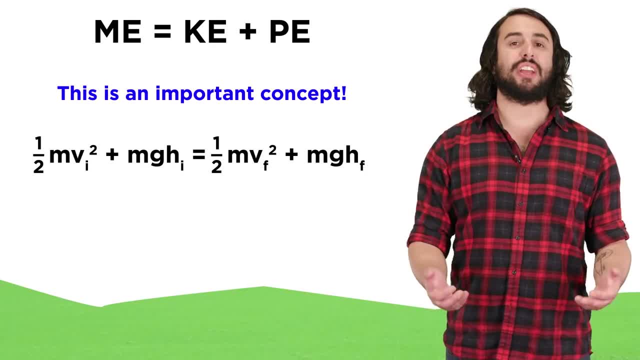 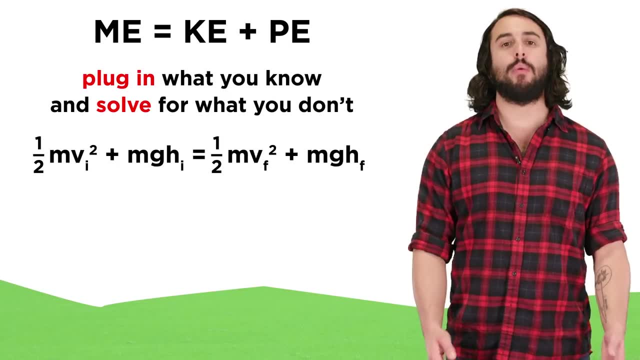 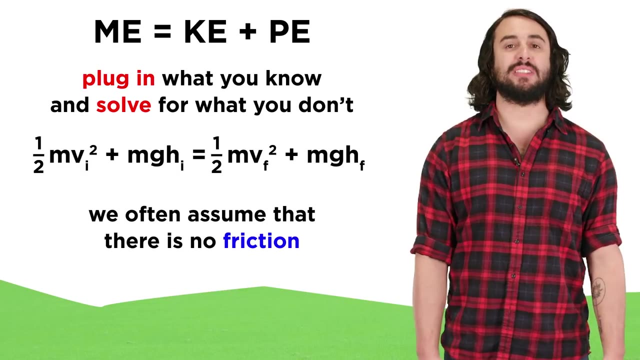 This equation will be used frequently in physics when we want to assess the kinetic or potential energy of an object at a particular moment, and if we have enough information about a system, we will be able to algebraically solve. for some unknown, This only works when there is no friction present, but for systems like a swinging pendulum. 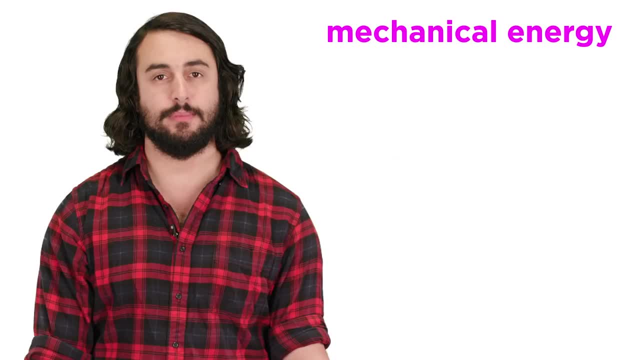 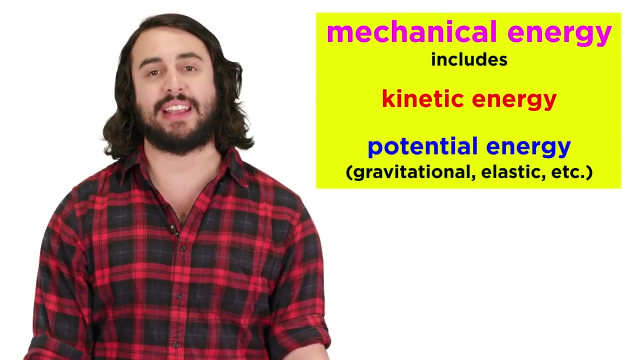 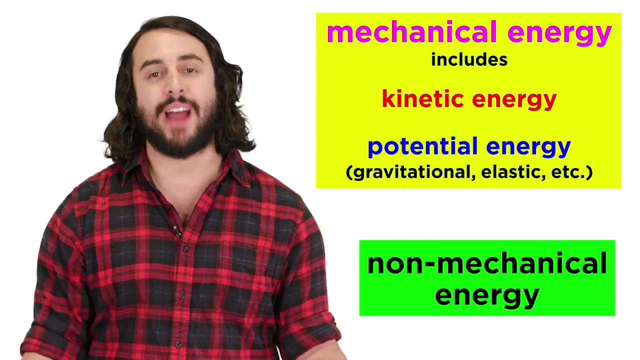 we can use it anyway, as the force of friction will be negligible. Once again, the label of mechanical energy is just a way of categorizing energy. It distinguishes kinetic energy of motion and gravitational or elastic potential energy from other forms of energy which we call non-mechanical energy. 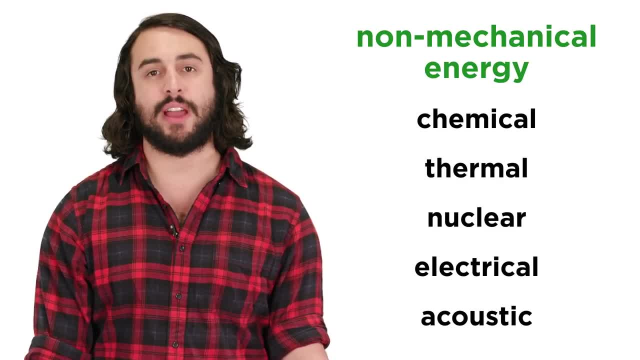 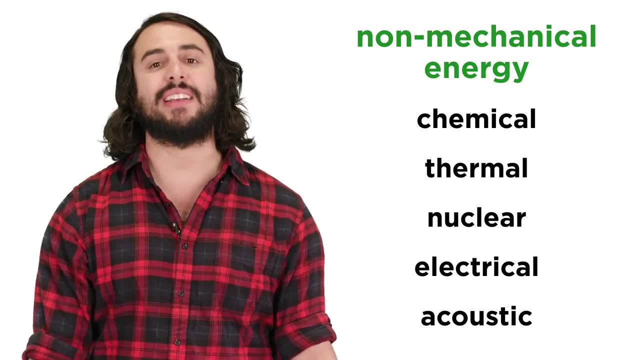 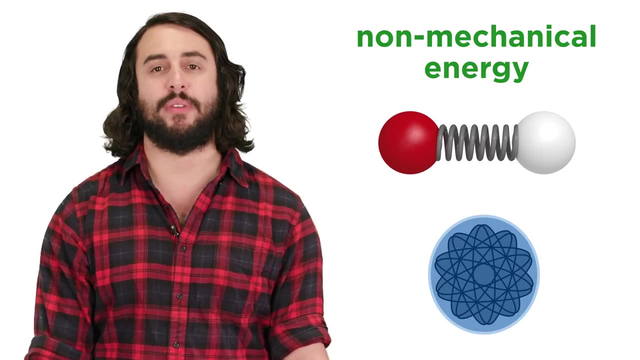 This includes things like chemical energy, thermal energy, nuclear energy, electrical energy, acoustic energy, electrical energy- These are also some kind of kinetic or potential energy, as they involve the motion of tiny vibrating particles, the energy stored in an atomic nucleus or some other form of energy. 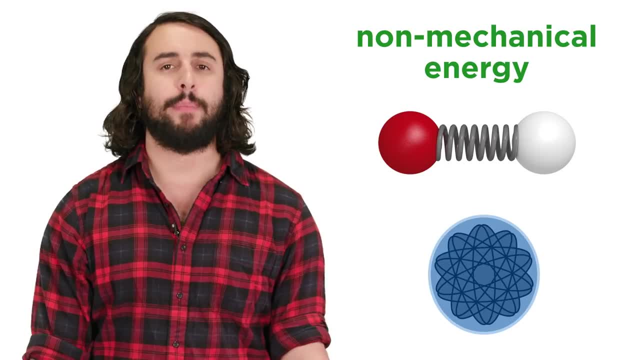 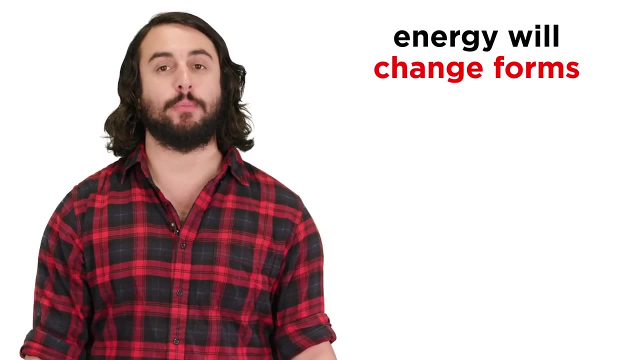 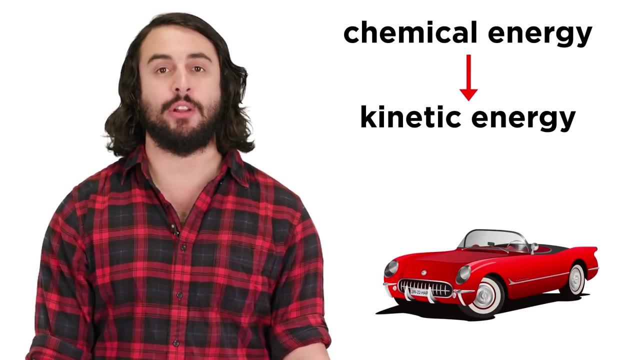 associated with either motion or storage, But they differ in nature from mechanical energy. As we said, energy can be transformed from one form to another, but it is always conserved. A car engine converts chemical energy stored in gasoline into energy. The car engine can be transformed from one form to another, but it is always conserved. 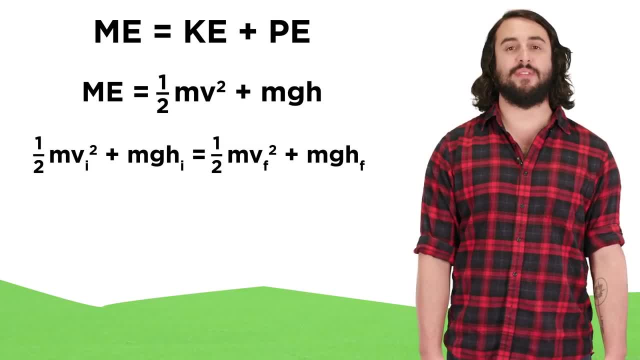 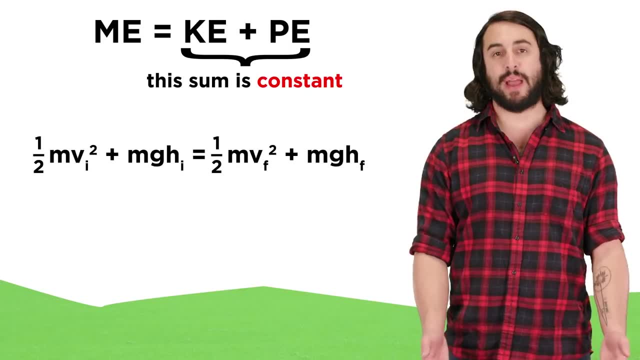 initial plus mgh initial will be equal to one half mv-squared final plus mgh final. It shows that the sum of the kinetic and potential energies of a system like the pendulum will be the same at every point in its motion. 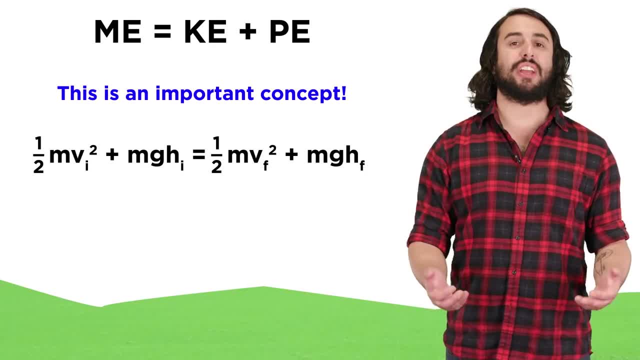 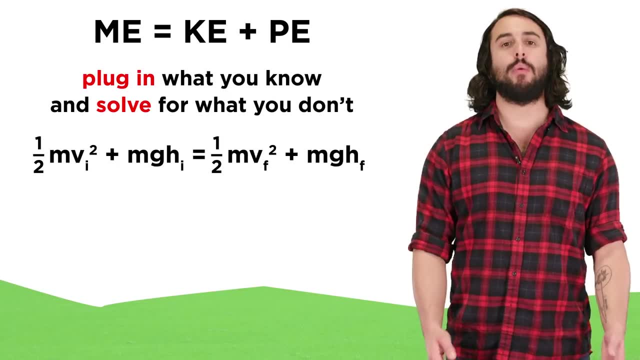 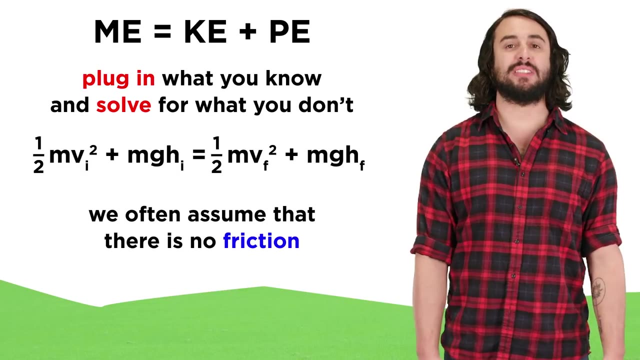 This equation will be used frequently in physics when we want to assess the kinetic or potential energy of an object at a particular moment, and if we have enough information about a system, we will be able to algebraically solve. for some unknown, This only works when there is no friction present, but for systems like a swinging pendulum. 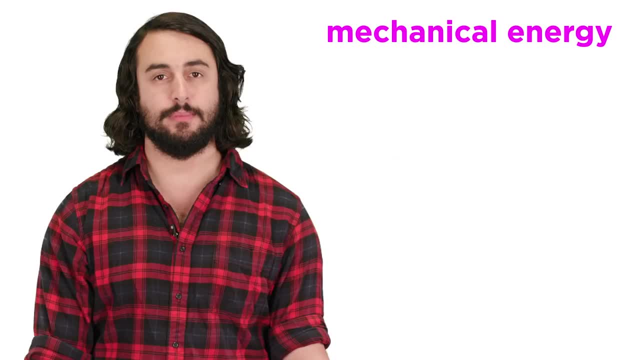 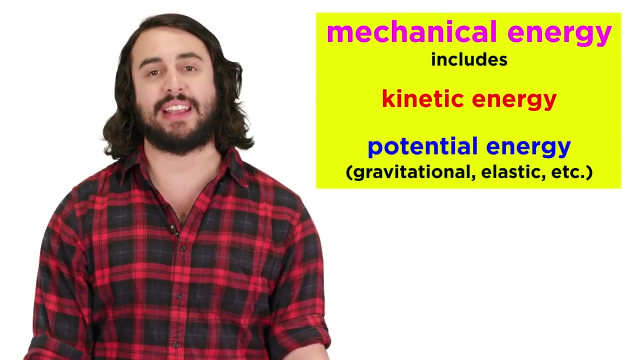 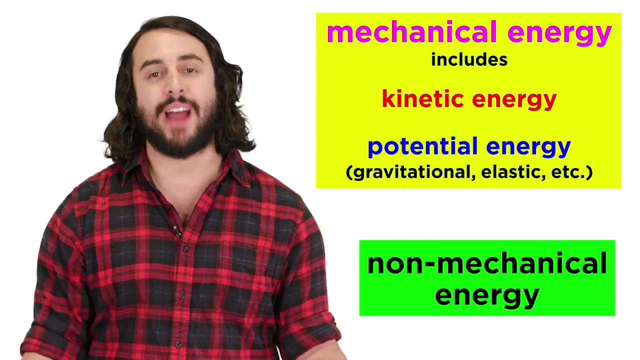 we can use it anyway, as the force of friction will be negligible. Once again, the label of mechanical energy is just a way of categorizing energy. It distinguishes kinetic energy of motion and gravitational or elastic potential energy from other forms of energy which we call non-mechanical energy. 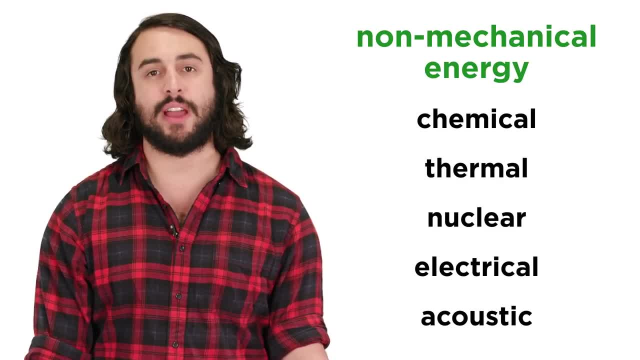 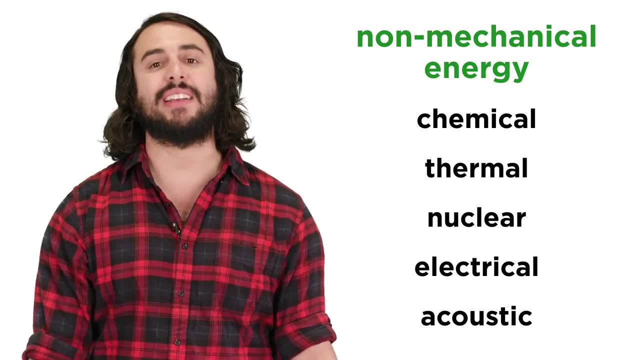 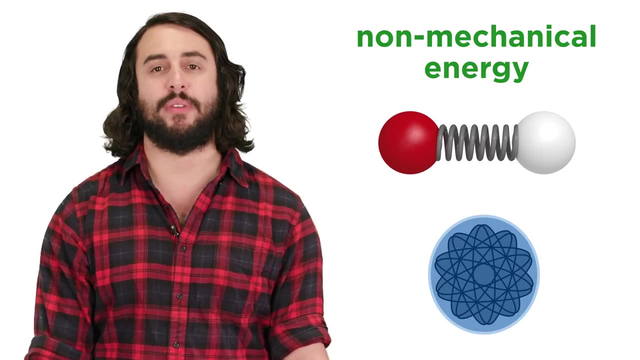 This includes things like chemical energy, thermal energy, nuclear energy, electrical energy, acoustic energy, electrical energy- These are also some kind of kinetic or potential energy, as they involve the motion of tiny vibrating particles, the energy stored in an atomic nucleus or some other form of energy. 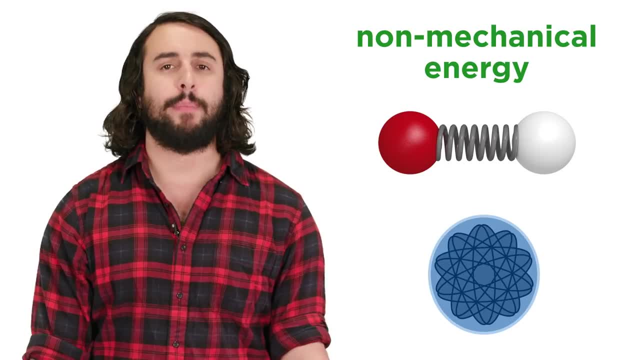 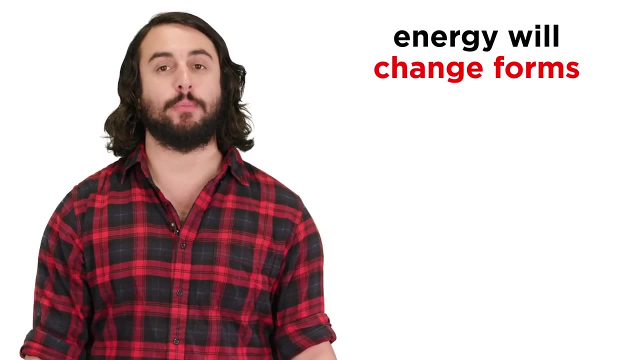 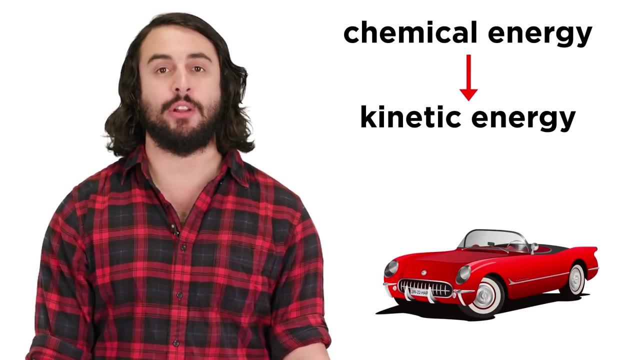 associated with either motion or storage, But they differ in nature from mechanical energy. As we said, energy can be transformed from one form to another, but it is always conserved. A car engine converts chemical energy stored in gasoline into energy. The car engine can be transformed from one form to another, but it is always conserved. 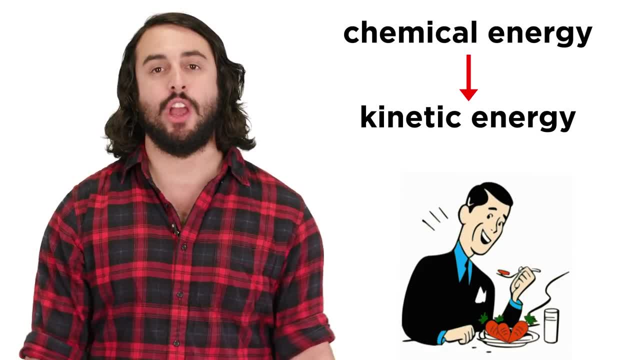 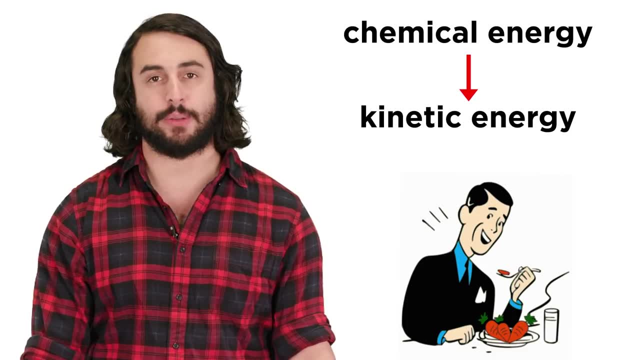 When we metabolize food, we are converting chemical energy within the food into the chemical energy in ATP, which can then be used as kinetic energy to move our bodies around. If, while moving around, you decide to slap your hand down on a table, all that kinetic. 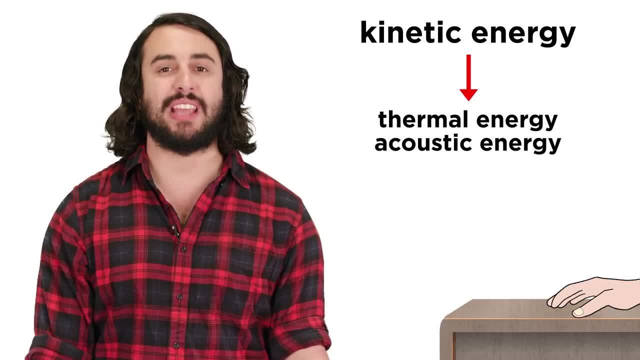 energy is transformed into thermal energy by heating up the table slightly, as well as acoustic energy, which is the sound we will hear when we move around the table. This is called kinetic energy. When we move around the table, all that kinetic energy is transformed into thermal energy. by heating up the table slightly, as well as acoustic energy, which is the sound we will hear when we move around the table slightly, as well as acoustic energy, which is the sound we will hear when we move around the table slightly, as well as acoustic energy, which. 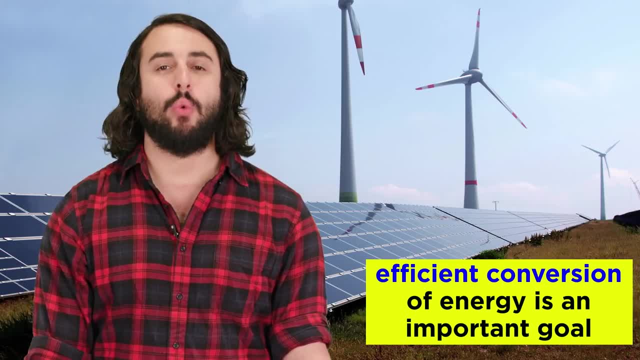 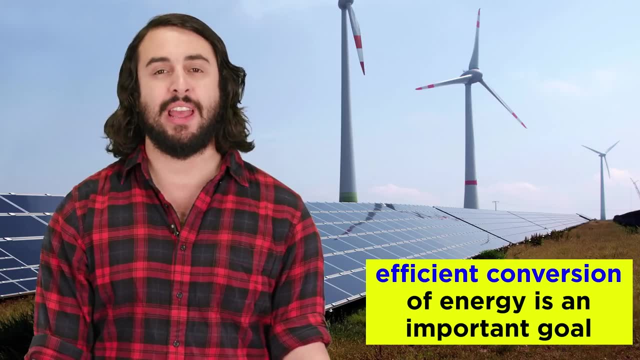 is the sound we will hear when we move around the table slightly, as well as acoustic energy. As we progress through the twenty-first century, we will continue to try to find more efficient ways to convert energy from natural sources like solar and wind energy into the energy.